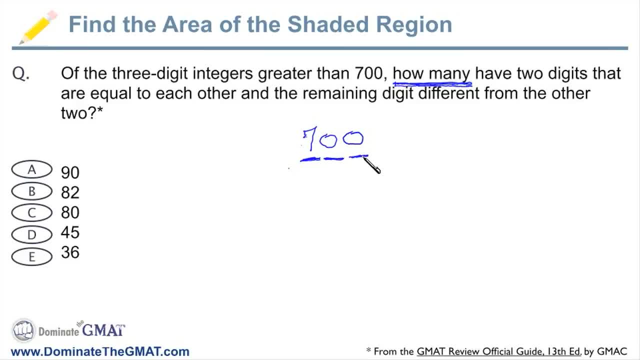 and then the units digit or the ones digit. that is that final number, And so we just want to be very clear on that. And then we have the hundreds place, which is the hundreds number, in this case seven, and then the tens digit, which is that middle number. 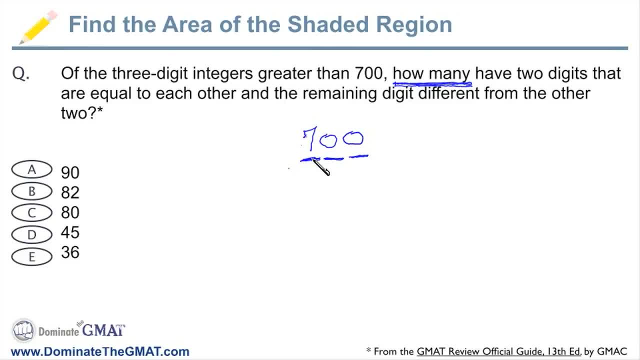 And so we're looking for ways that two of the digits are going to be the same and one digit is going to be different from each other, And there are really three combinations of that right. There are ways that the hundreds and the tens digit are going to be the same. 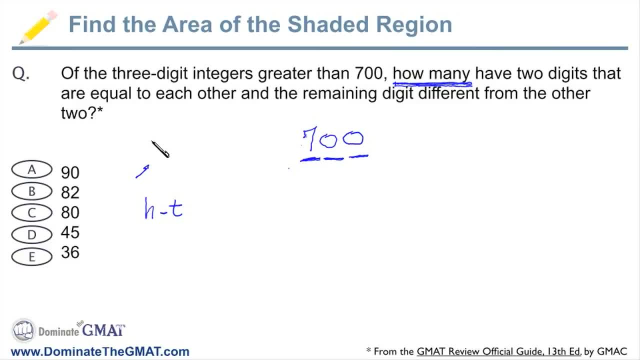 So, for example- I'll give you an example like 770, right, That would be a number where the hundreds digit and the tens digit is going to be the same. It's also conceivable that the tens digit and the ones digit is going to be the same. 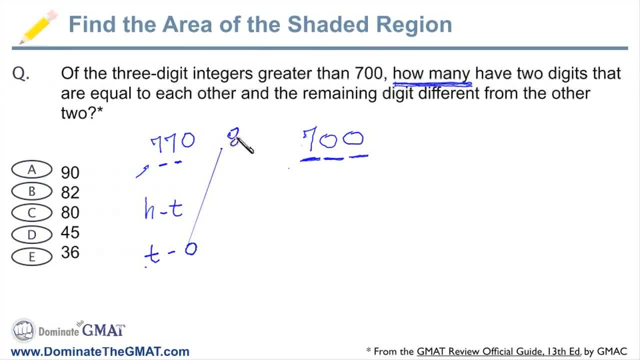 Right, That would be an example of like 844, right, The tens digit is the same and the ones digit is the same. And then, finally, we could have a scenario where we have the hundreds digit actually is the same as the ones digit. 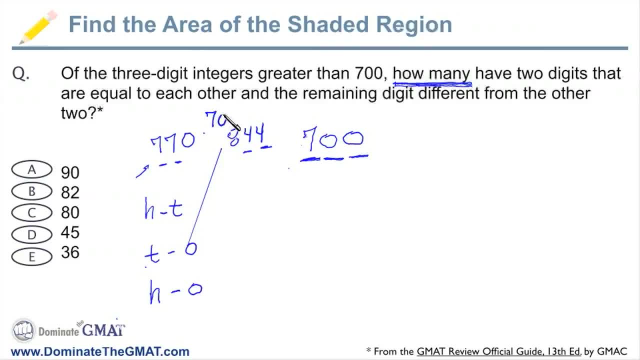 And that would be an example of like 707, or something like that, And so we're starting to make the list. Now the question is: how many of each of those combinations are there going to be? Well, we can further break it up. 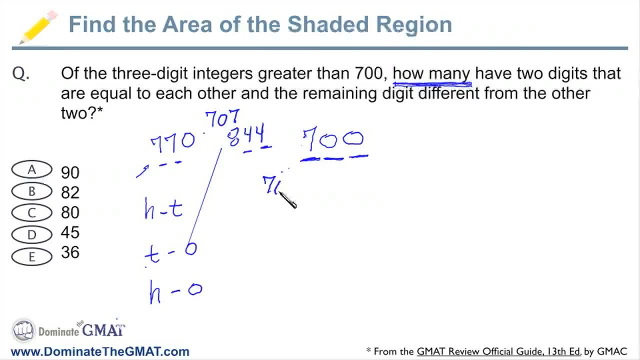 And think to ourselves: okay, certainly we have the 700s, And this is going to be the 700s to 799, right, How many times is it going to happen there? Because at that point we're going to kind of tip over into the 800s. 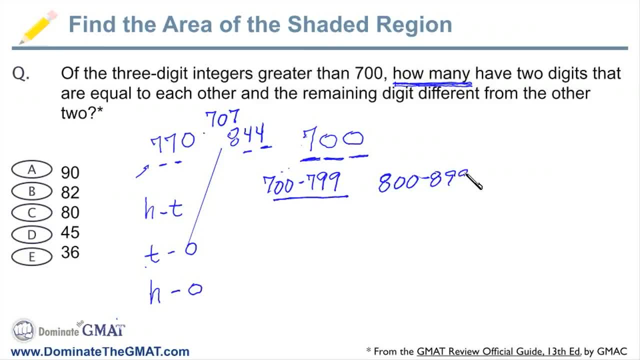 We're going to go 800 to 899,, right, And then, finally, we ultimately are going to have the 900s to the 999s, Because it says how many are there going to be starting at 700, but we're looking at three different integers. 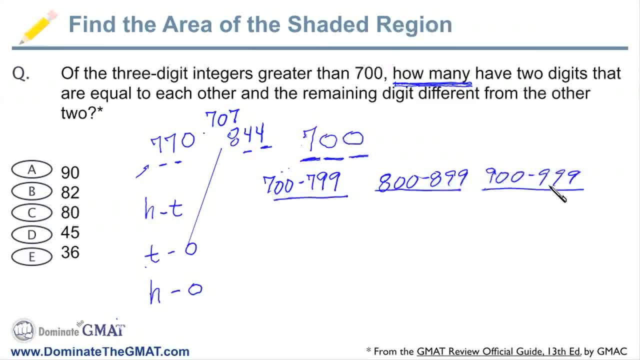 So once we get to 1,000, we no longer have 390.. We're going to have three digit integers, And then it's just a matter of literally thinking through it, right? So let's start down here. I mean, what do we have? 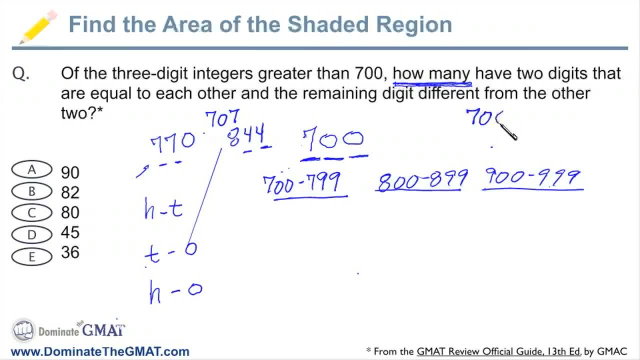 The hundreds and the one, for example. So we have 700.. What does that tell us? Well, in that case it says greater than 700.. So that actually doesn't count. The 00 doesn't count, But we could have 707,, for example. 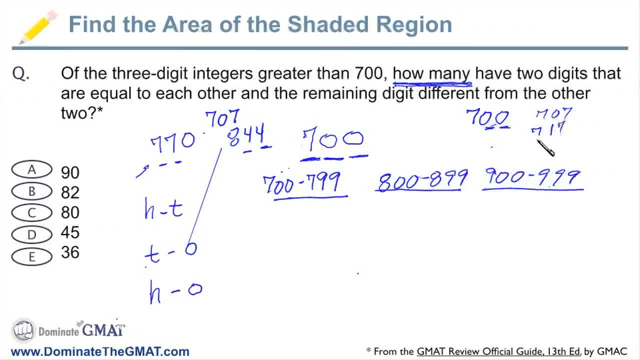 And then we could have 717.. And then 727, right, And you start to recognize the pattern. Well, how many of those are there going to be 737, 747?? There would be 10 of them, right. 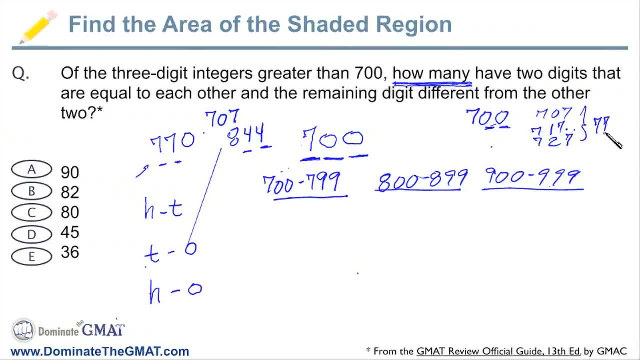 Ah, except we don't want to count 777. Because that and all three are the same. So if you think about it, between 700 and 800, there are going to be nine instances where the hundreds digit and the units digit. 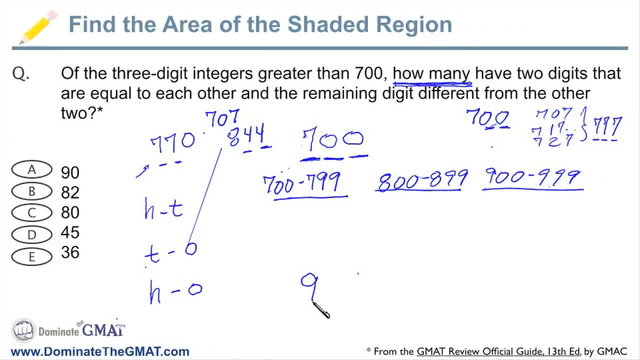 or the ones digit is going to be the same, Because 777 doesn't count. And then you start to recognize a pattern. Isn't that going to be the case all the way across the board? It's going to be the same in the 800s, right. 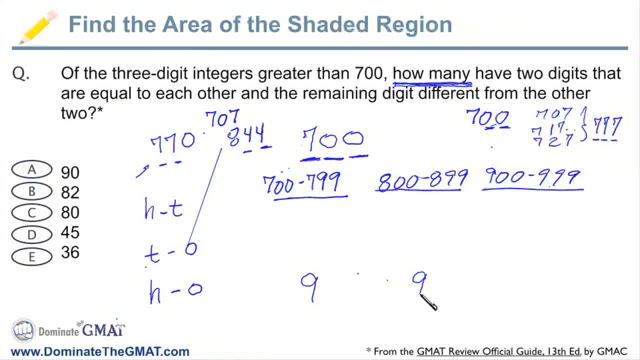 808, 818, 828, 838, 848.. Ten of them, except we don't count 888, so we have to subtract one, so there's really only nine. And then the same thing up here, right. 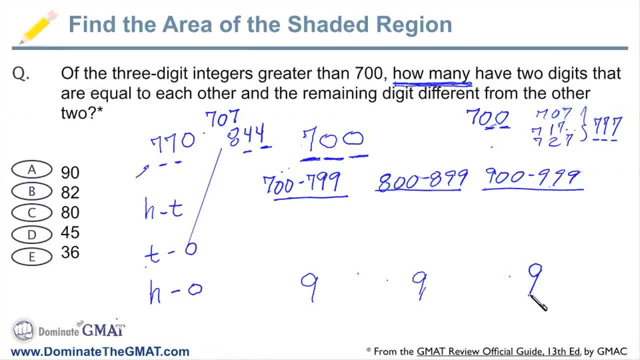 We have 909, 919, 929.. The one that we accept is 999, because that's all three the same and we don't want that. Now, is this pattern going to apply for the tens and the ones? Well, let's look. 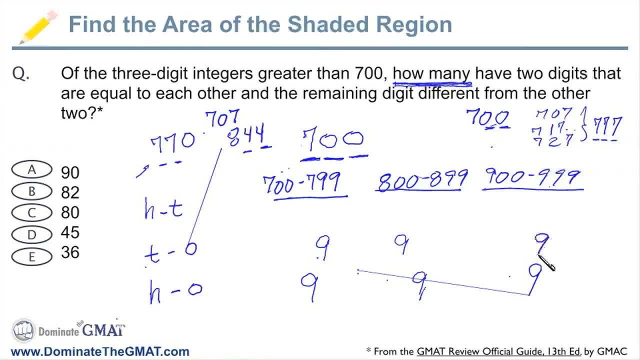 You know, we just have to confirm it. For the tens and the ones. would we have 999?? Well, we would have 700.. Well, that doesn't count. How about 711?? How about 722, 733,, 744, 755?? 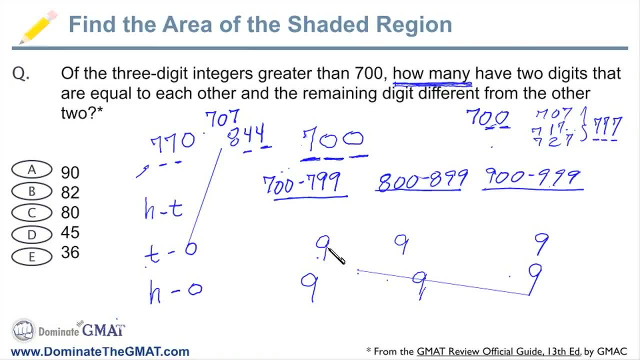 Well, we would have to subtract 777, so there would be nine. Now look, 700 itself isn't going to count, because the question says greater than 700. So actually, we're not going to have nine In this instance, we're going to only have eight. 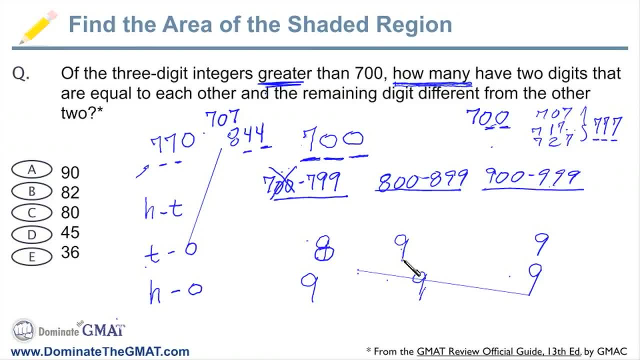 But we would have nine here, right, Because 800 counts, because that's greater than 700.. 811, 822, 833, 844, and so forth, except 888, that doesn't count. So there are going to be nine of those. 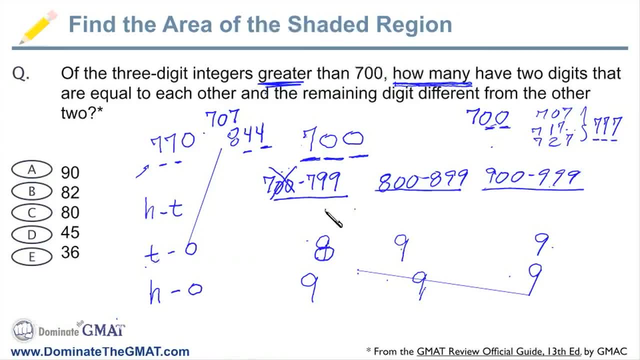 There are going to be nine of these. And how about the hundreds and the tens? We have 770, 771, 772,, 773, 774, everything except for 777.. So there's going to be nine of those. 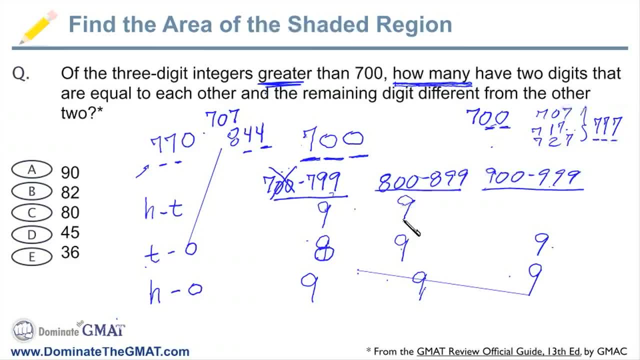 Sure enough, the same thing here. Nine of those right, Because 800,, 811,, 822,, 8.. Oh, sorry, And the tens So 880,, 881,, 882, and so forth, And there's going to be nine of these. 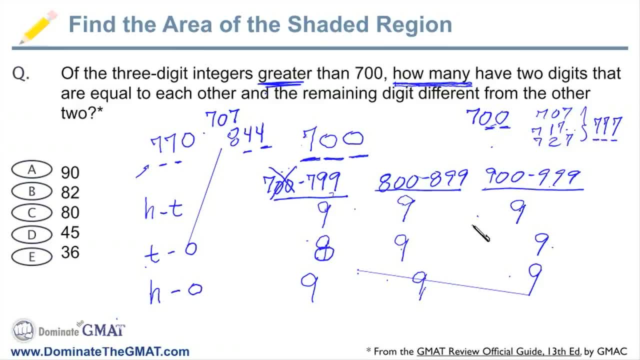 So we're going to be able to pick this up relatively quickly. In fact, you can see that the total number of numbers, for which two of the digits are going to be the same and one is going to be different, is just going to be nine times. 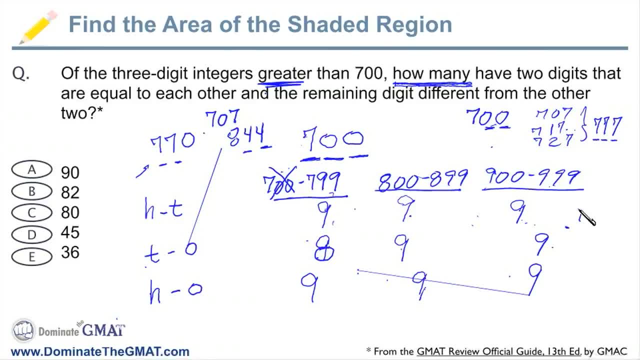 How many are there? Nine, nine, nine, Nine times nine, right. Nine times nine is 81.. Except that's not one of our answer choices, because what do we notice? In one instance we have one fewer. We have to account for the fact that the question says: 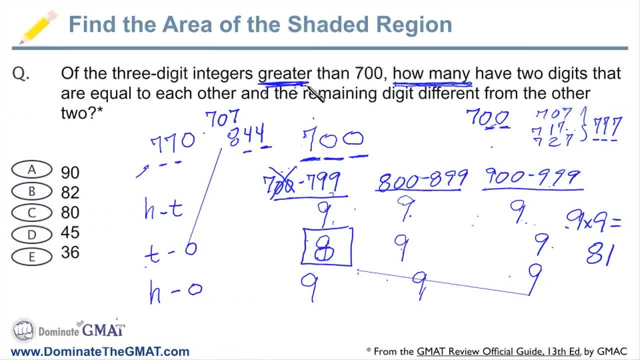 greater than, not greater and equal to, but greater than, And so it's going to be 81 minus, Sorry, minus the one or 80 total. And so when we look over here at our answer choices, Bingo, We have 80 is correct. 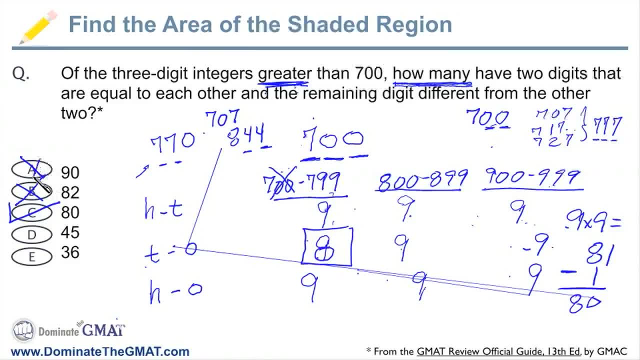 82 is close if you did something a little bit wrong and then 90 is just flat out wrong. 90 would be the common wrong answer. if you put 10 in each one of these boxes, Like if you thought it was 10,, 10,, 10. 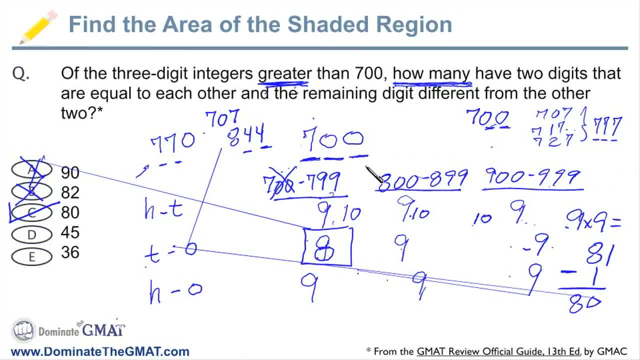 you'd probably come up with 90 as your answer, but again we have to account for the fact that 777,, 888,, 999- those numbers don't count because all three digits are the same and the question only wants two of them to be the same. 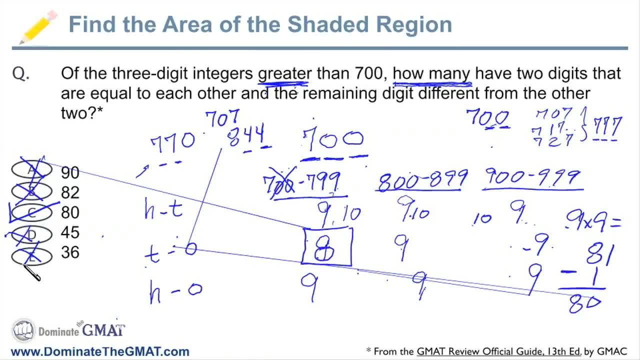 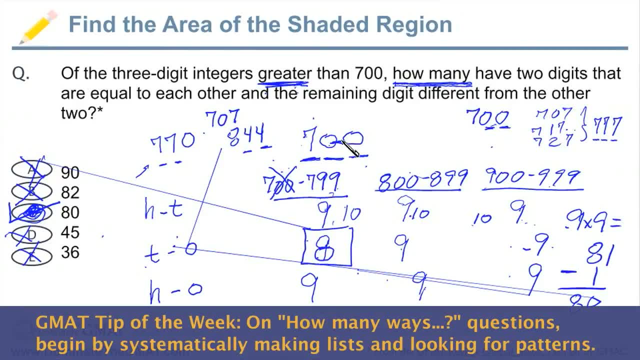 And if you pick D or E, you just flat out missed something. So the correct answer is C. Good job if you got that. and again, the tip is when you see questions that ask: how many right, How many different ways of doing something are there. often times, if you just